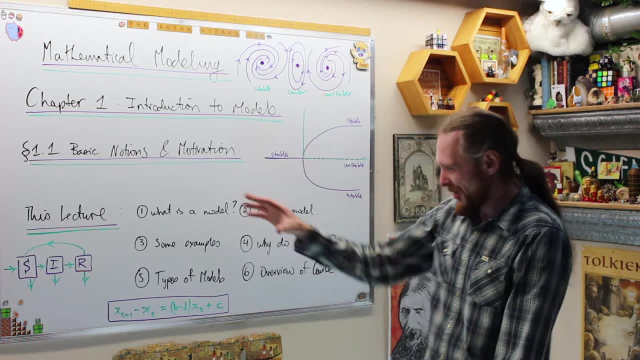 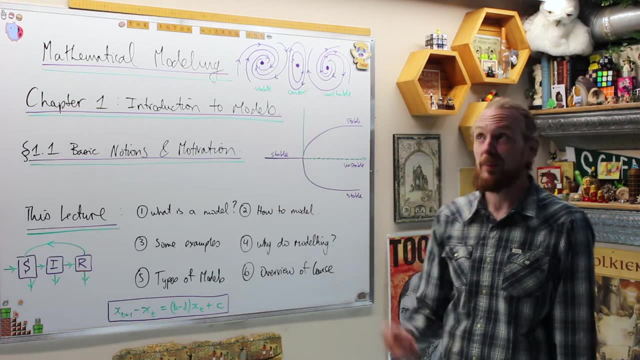 what we're going to discuss here, And then we're going to give an overview of once we have an idea of what a model is and how we're going to do it. We'll give an overview of what the rest of the course will be, what chapter two, three, four, five and possibly six will be in this playlist. 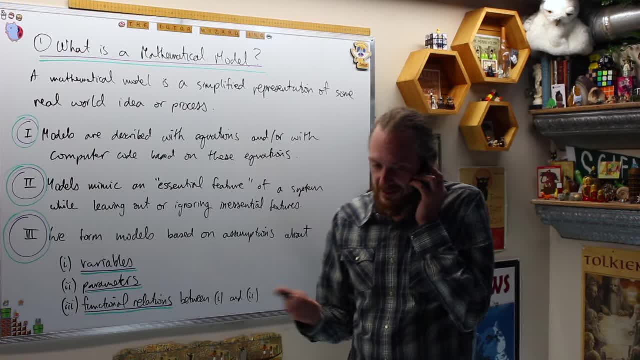 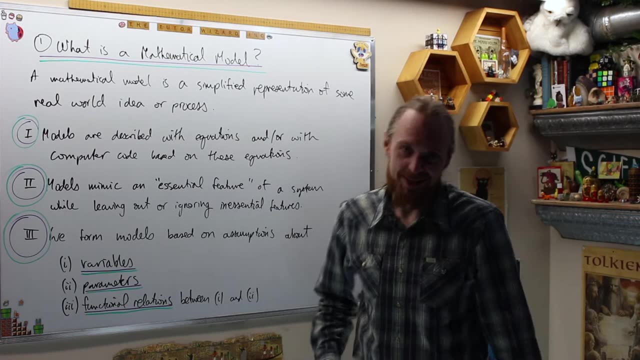 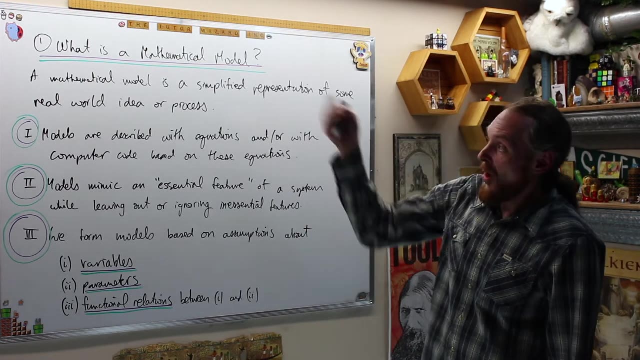 Let's get to it, All right, Mark? Yeah, send me, I'll watch some and then I'll email you back tomorrow. Okay, Bye, Solomonovitch on the phone, Leave me alone. We're doing videos, All right, That's another one. Linear algebra coordination- What are we going to do? One: 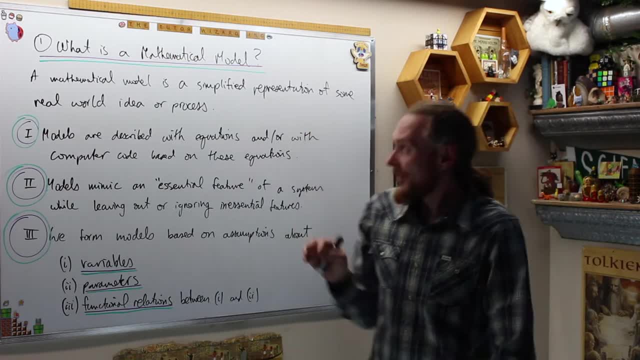 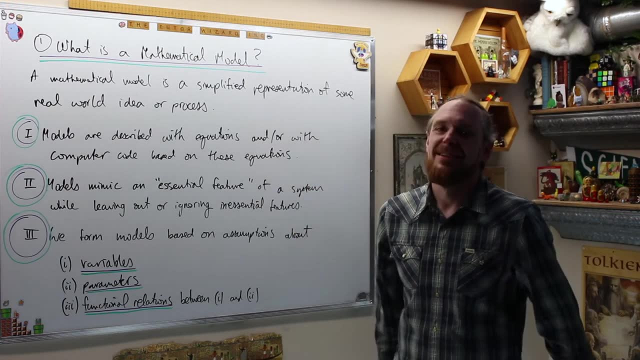 what is a mathematical model? A mathematical model is essentially a simplified representation of a real world idea or process. The clever joke or the classic quote is: I don't know who did it, Someone wiser than me. No models are correct. Some are more useful than others. 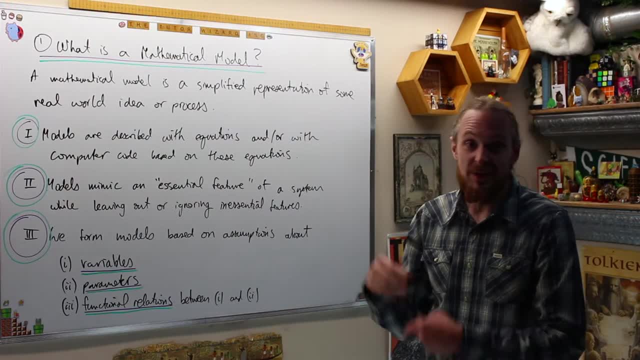 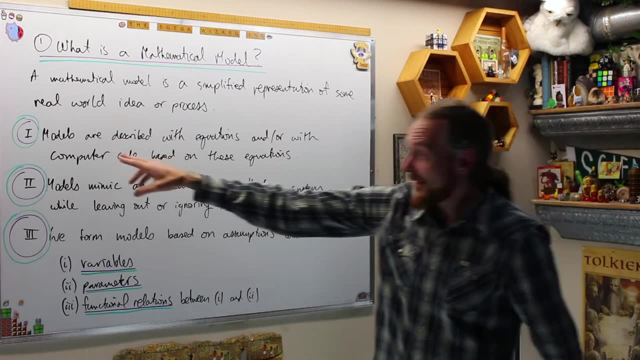 Simplifying and idealizing a lot of scenarios, but we're trying to get. we want to understand how a process works in the real world And we're going to use mathematical models, which means essentially mathematical models are going to be described with equations and or computer code. 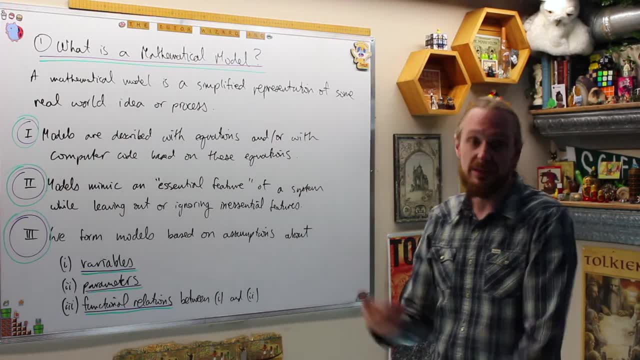 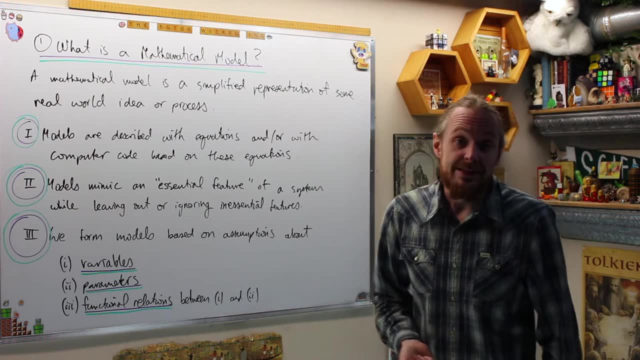 Once we have those equations we can put them into computers and let them do all kinds of different simulations based on that And then get ideas of how to. for instance, my running model will be spread of infectious disease. So if we want to know how disease changes, we try to model. 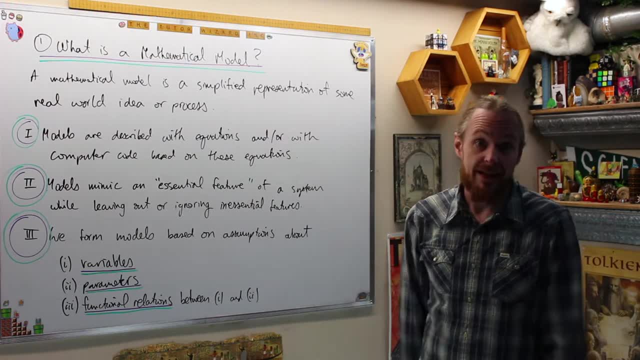 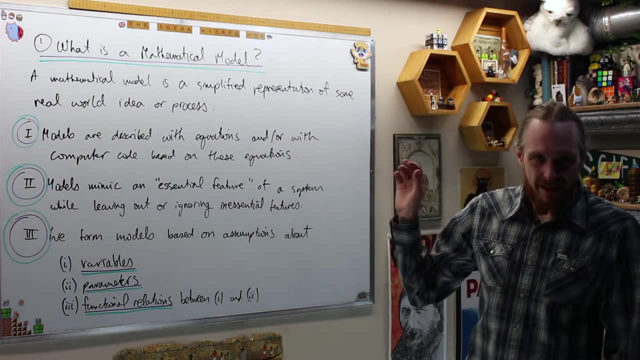 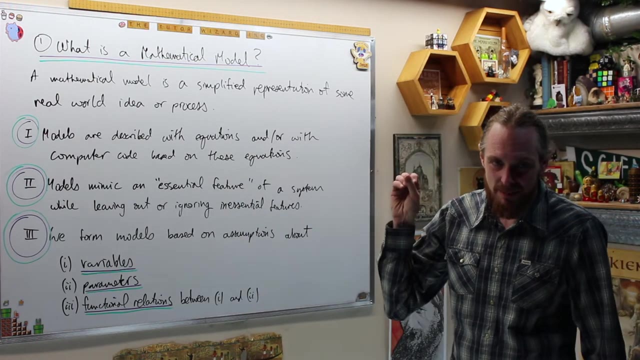 that with some equations, And then we want to eventually analyze and see how we can mitigate that disease or stop that disease from spreading. A model also mimics a good idea is and number two. number two is basically giving us the caution to not making your model the most sophisticated. 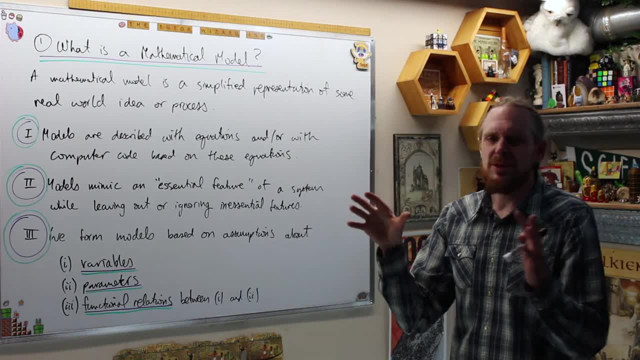 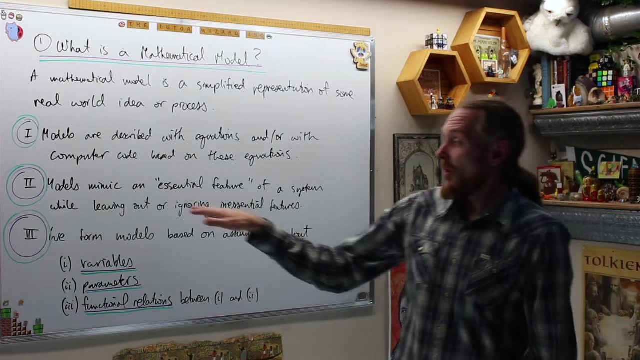 or the most like the real world a lot of the time, because then it will just become so complicated and convoluted as to not being able to solve or get any distill anything meaningful out of it. So what we're going to do is we're going to mimic the whatever we're going to call the essential. 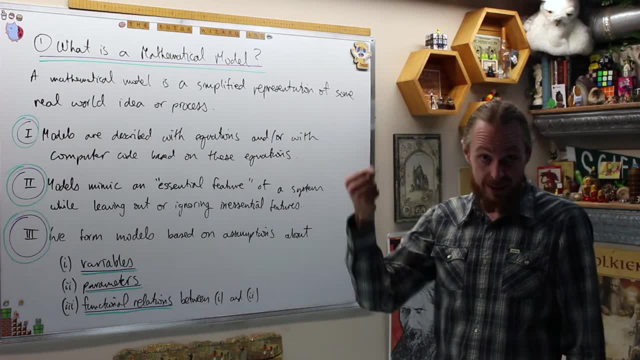 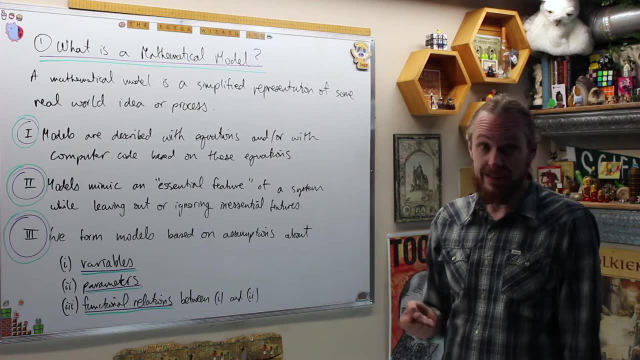 features of a model. specifically, like quite often when we do spread of disease, I'm going to focus on the infected individuals And there will be other components in there, but we will focus less on those. we're just going to focus on the infected individuals and then try to get an explicit 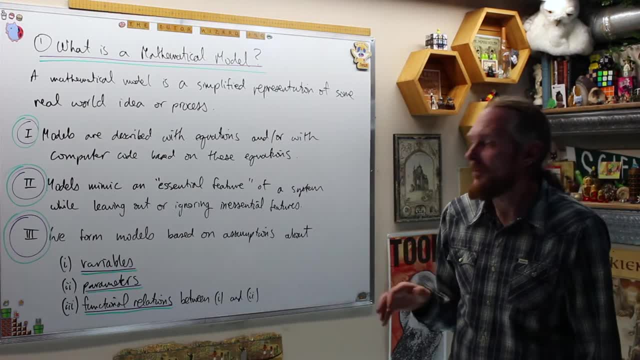 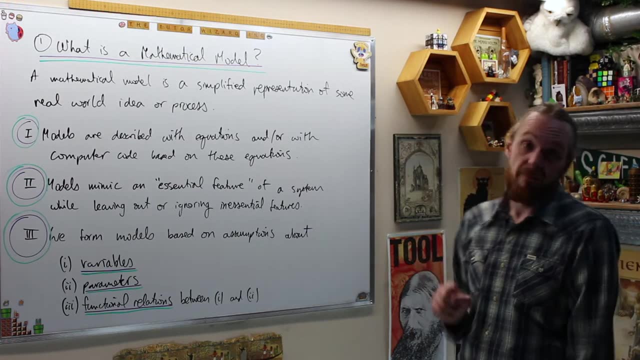 solution to those models. What else do we do with models? Basically, how are we going to start forming the models? we're going to form the models using variables, parameters and functional elements between those variables and parameters. What are the variables? Obviously, those are. 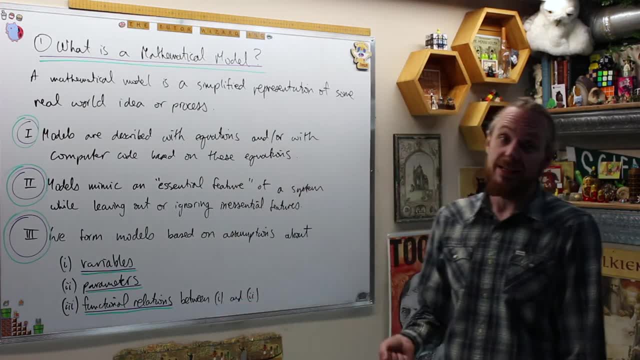 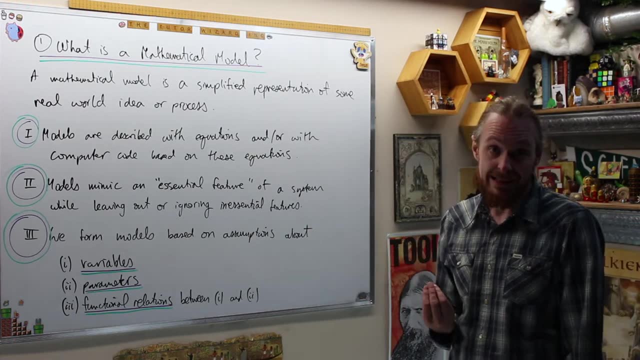 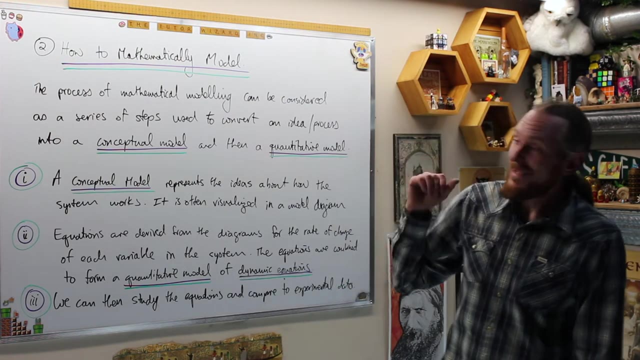 things that vary or change over time And the parameters are going to be things that we will have to sometimes search for a parameter fix. But once we do that, they are fixed constants in the equation, Let's do the next. point Two is going to be discussing how do we actually mathematically 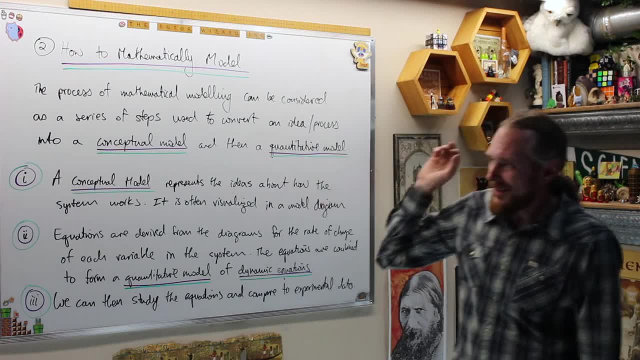 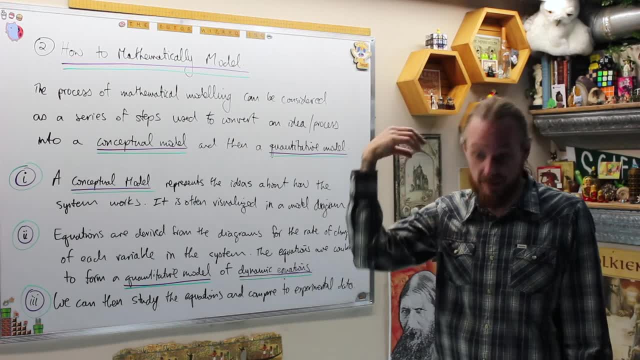 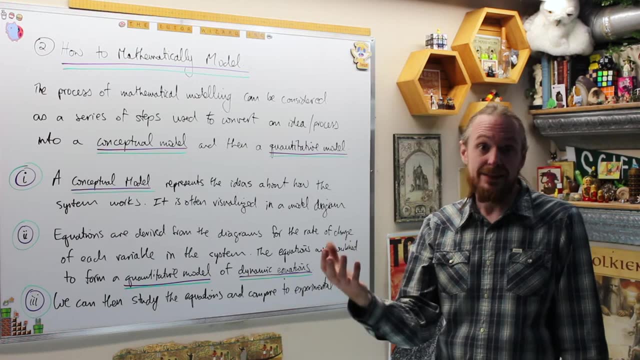 which is going to convert. the idea that we want to focus on in the one that I always run, is how to mathematically model the spread of infectious diseases. So how do we know how many people are infected in a given population? This is the question we constantly want to know. We're going 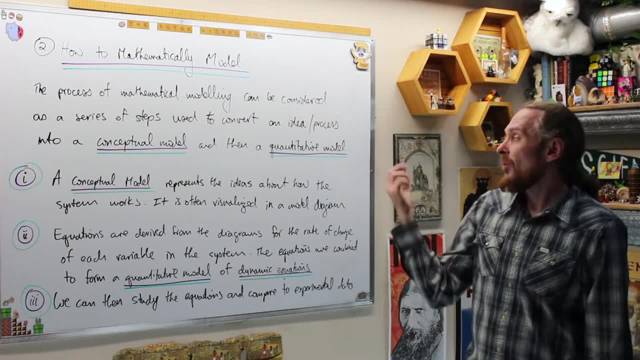 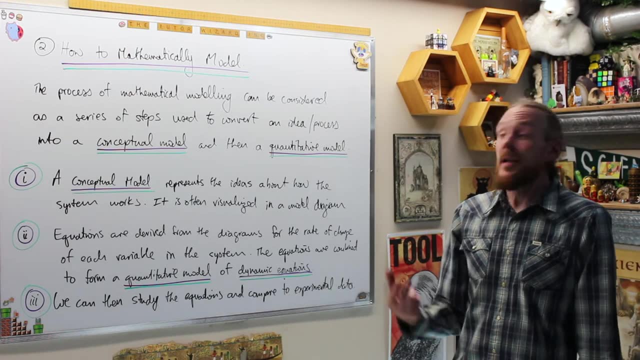 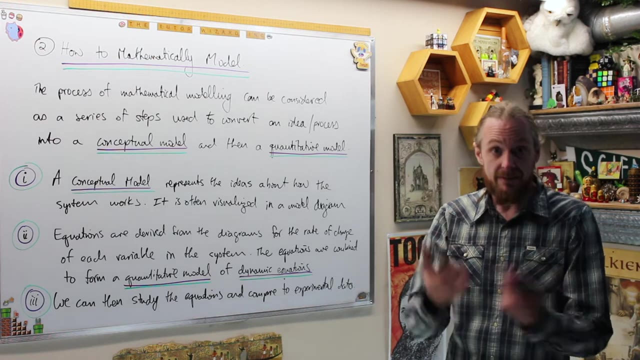 to go from that conceptual model to a quantitative model. The quantitative model will be equations either in discrete time or continuous time, And what that's going to allow us to do is eventually analyze the model of the scenario and make predictions about future and past behavior of the process. 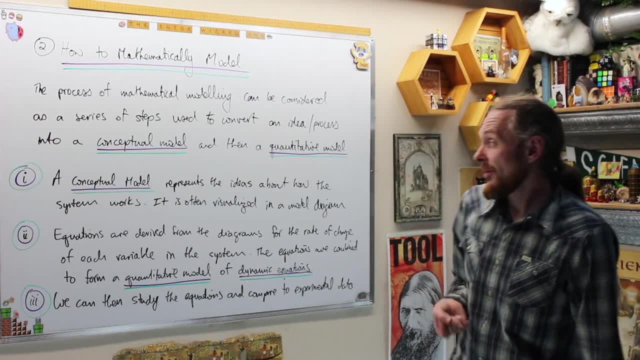 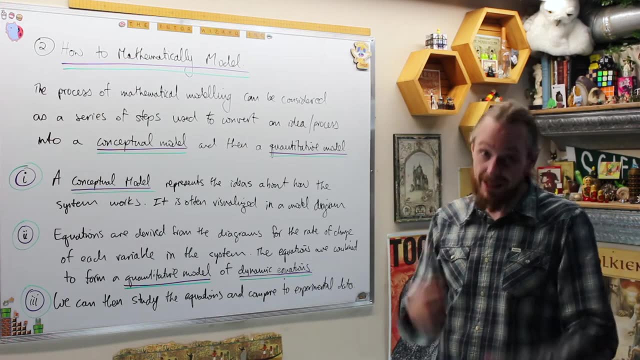 that we're interested in. So the conceptual model is going to be representation of the ideas of how we think the system actually works, And then we're going to make a bunch of assumptions or sit down and put a bunch of brains together and try to figure out how we think that that thing works. 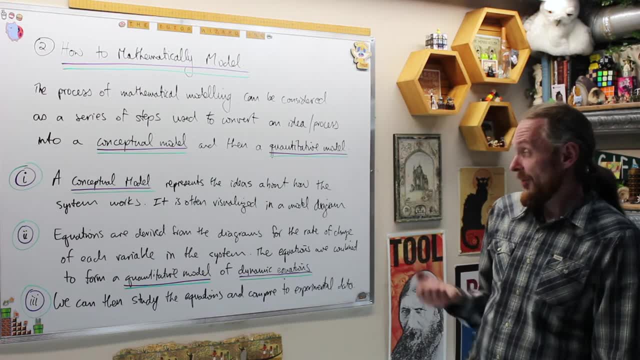 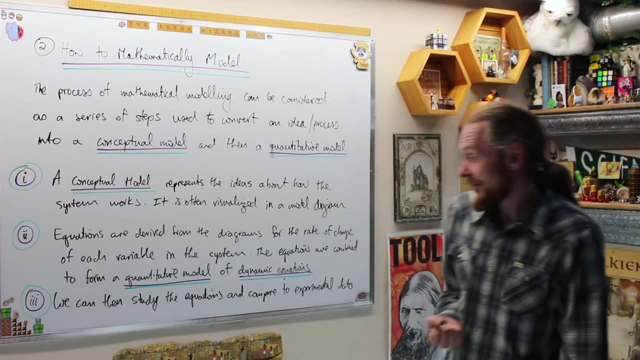 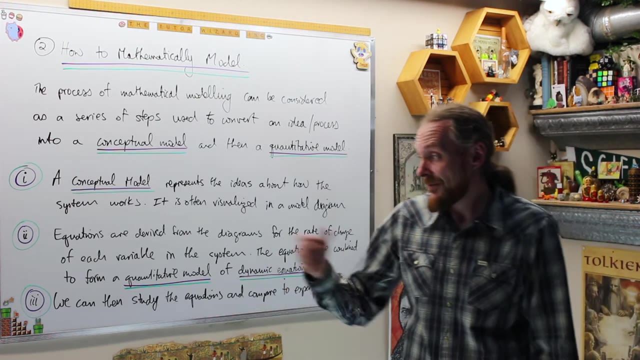 Then we often use visualization in the form of model diagrams or compartmental diagrams. From those compartmental diagrams we derive equations And then we specifically have the equations that are going to involve the rate of change of each of the variables in that system In the spread of disease. we're going to have quite 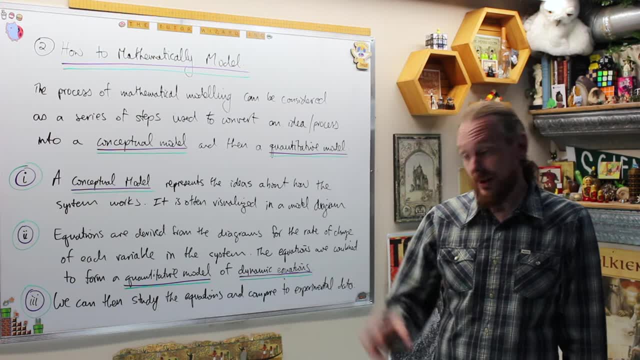 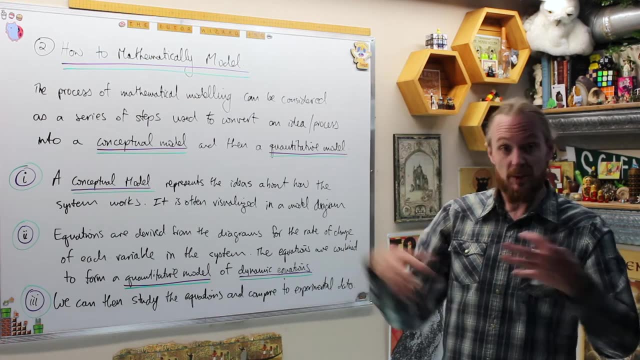 often susceptible categories, infected categories and recovered categories of people. So then we have an S and an I and an R, And those are our three variables And they're all changing. All those populations of people are changing over time And we want to derive some kind of difference or 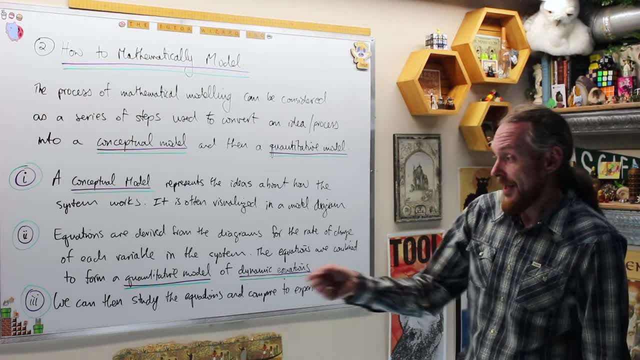 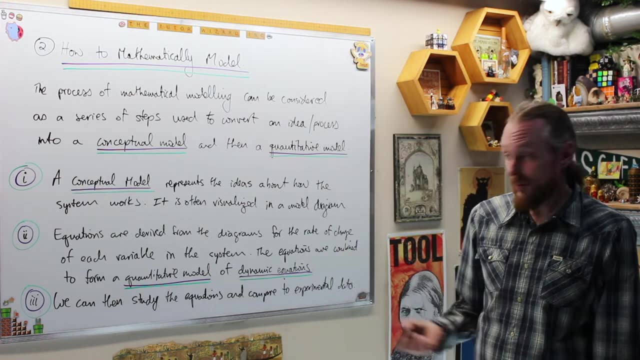 differential equations to describe those populations. And then, of course, once we've done that and we get good at going from the conceptual model to the quantitative model, which consists of a bunch of dynamical equations, once we do that, we really 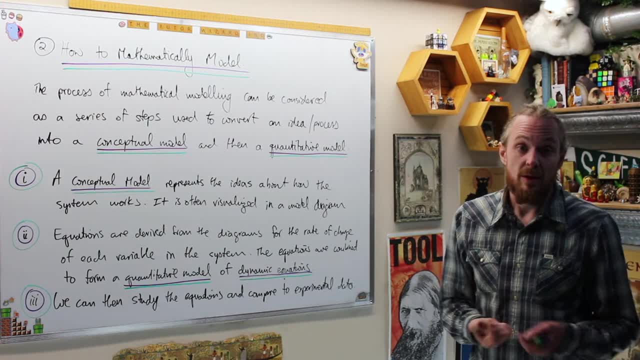 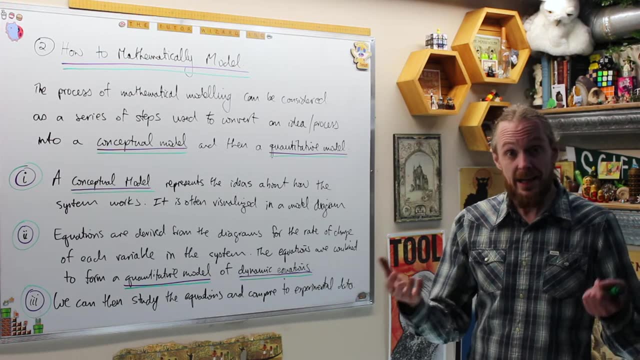 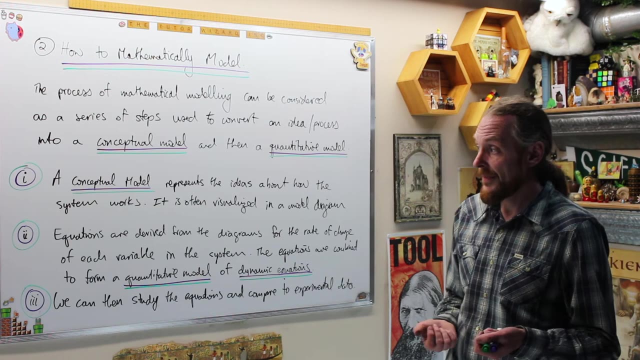 want to start studying and analyzing the long-term behavior of those solutions to those models And that will give us ways of doing quarantine or vaccination, say, for specific diseases, so that we can actually mitigate in a meaningful manner those infectious diseases. All right, let's do three. 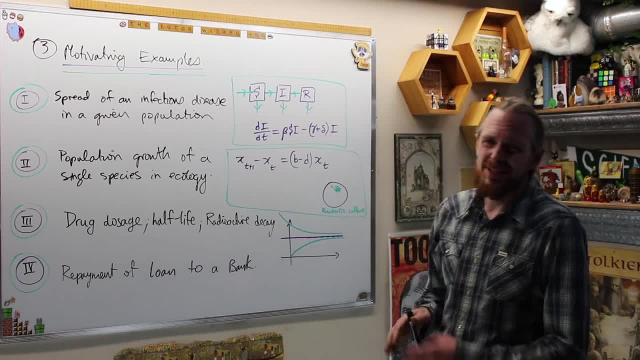 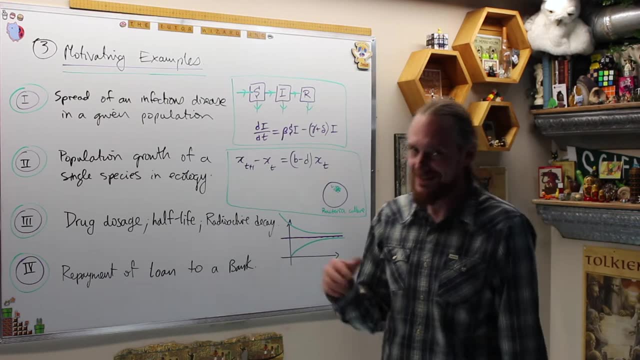 All right. three is motivating examples. I'm just going to list them. We'll try not to, but already you'll see I'm going to start explaining how everything works. We'll get to that in later videos. You'll see when we get to the gory detail. But the spread of infectious diseases in a given 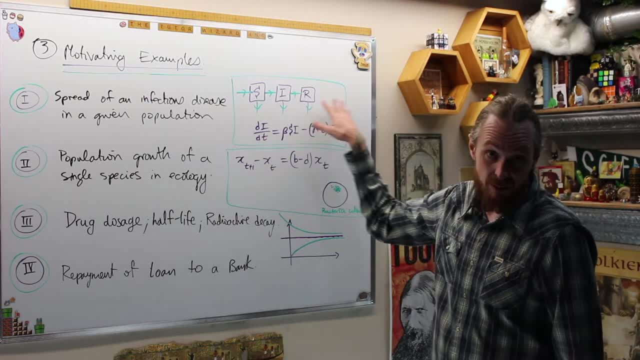 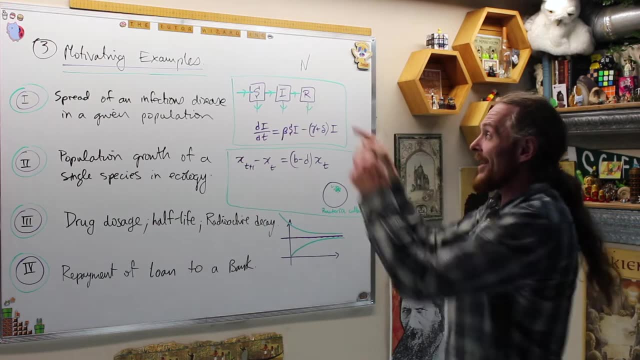 population. what we classically do is- or you'll see, we're going to do a whole bunch of videos on this- First, what we're going to do is just assume that the population is going to be a total population N, and then we're going to break it into two categories: susceptible people. 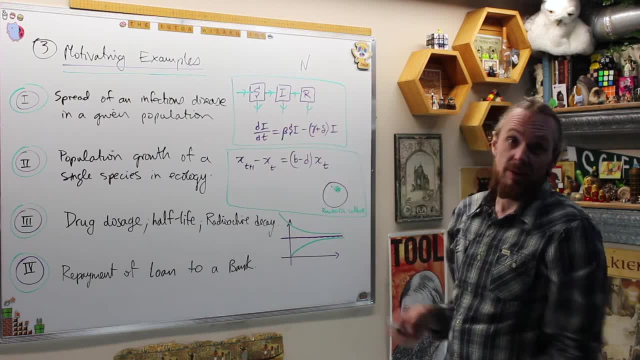 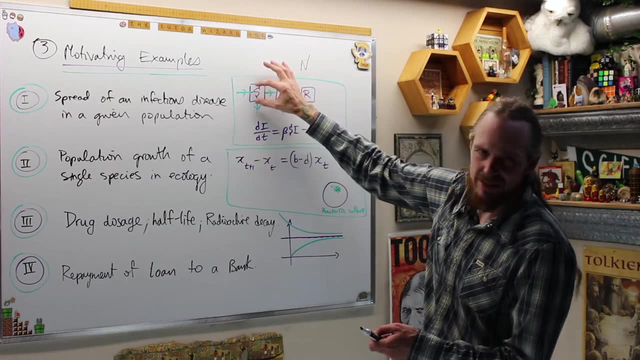 and infected people, And then what we're going to do is the diagrams that we were talking about in the last. in number two is the conceptual idea: is we make these compartments or the box that has the population of all these different kinds of people in there, And then we want to. 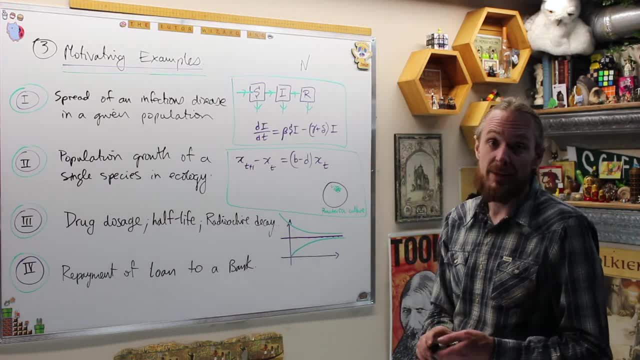 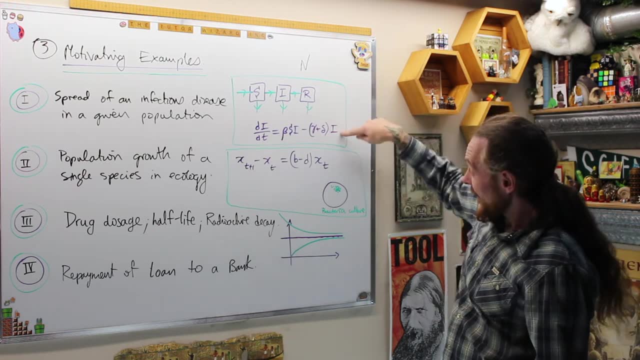 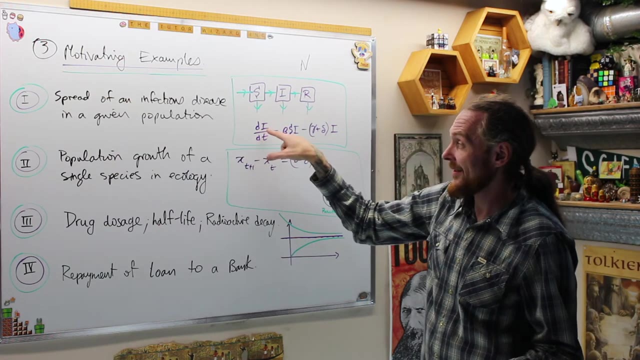 look at the rate of change of those populations over time And then from that diagram and once we label everything in the videos we can derive: this is the conceptual idea and this- this is the explicit equation or the quantitative modeling of the idea of how we think that the rate. 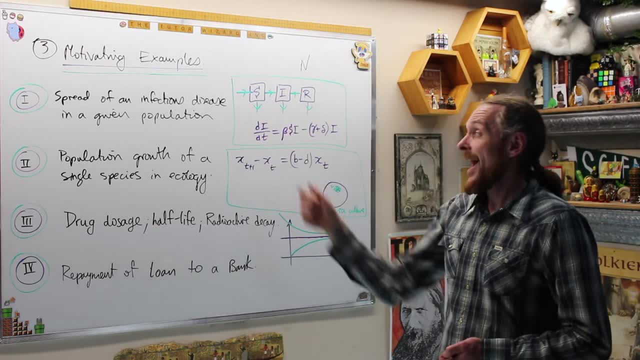 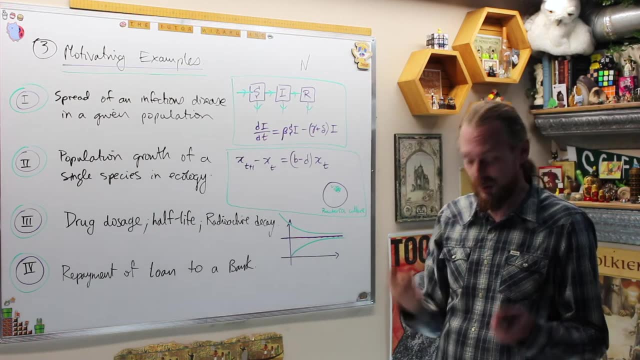 of change of I, which is the infected over time, which says how is the infected population changing over time. we think that this is the equation that describes that in certain models anyways, and we'll go through a whole demographic of a bunch of different SIR models. Another good one is: 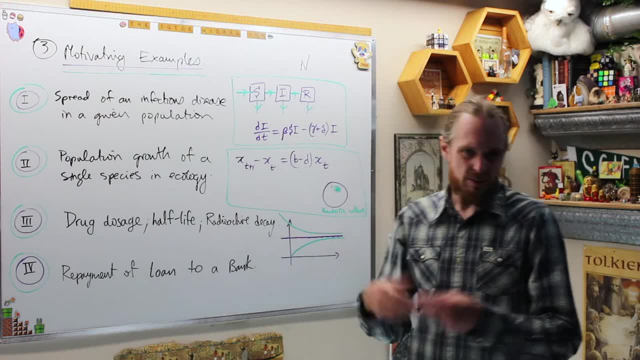 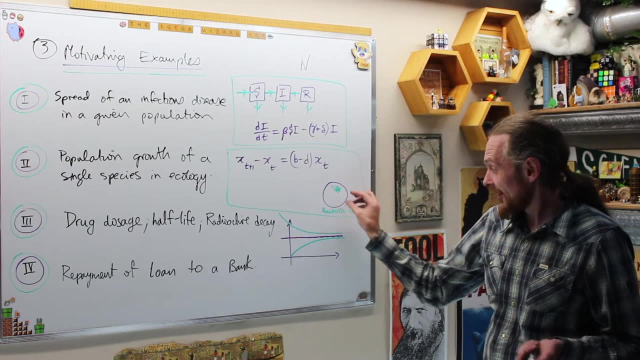 population growth of a single species in ecology or multiple species. we'll get into that also. But a good way of discreet time about that is if we have a bacteria culture of some kind and it starts off where we have some biomass in there And then we're going to check it every six hours or every 12 hours or once a day. 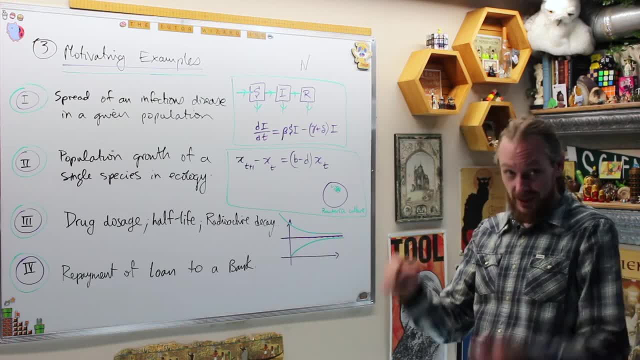 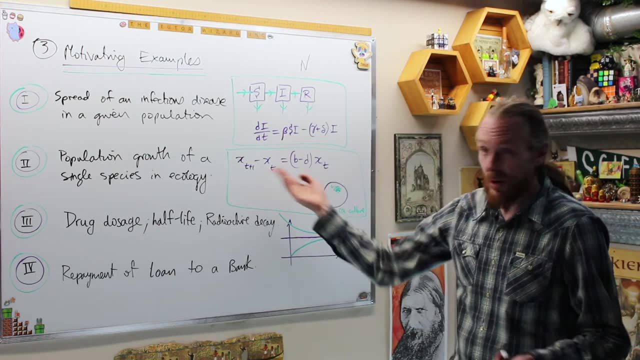 we go into the lab and I got to go in there and check and make sure I do my due diligence to do the experiment. we want to know how fast is that bacterial growth growing And one way to model that. So this will be a discrete time scenario. we're going to check it every day. So it's this. 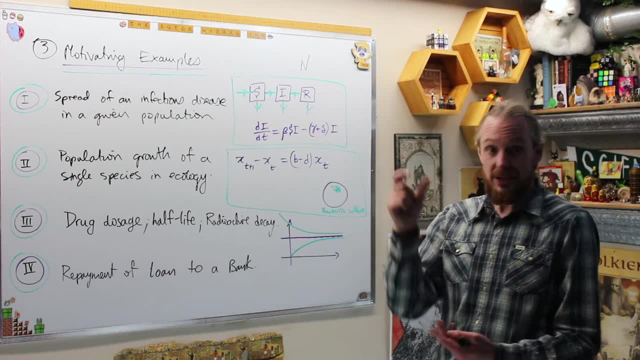 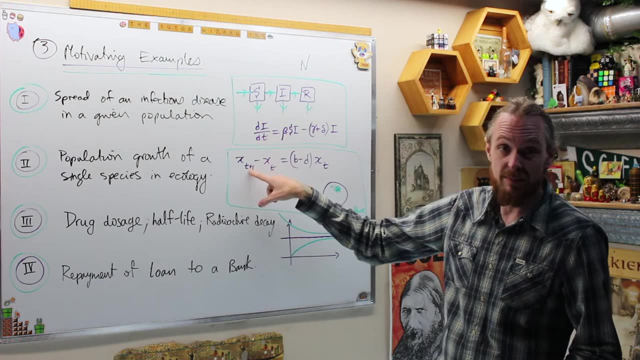 fixed length of intervals of time, And then we check it in those times And then we're going to do a little bit of time stamps, And so what that says is the difference between the original generation and the next generation, the difference between the two generations of the bacteria. 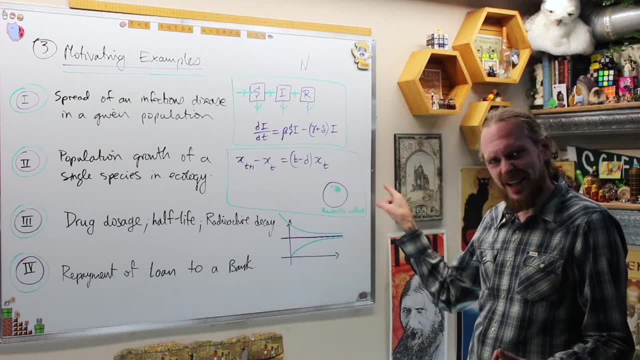 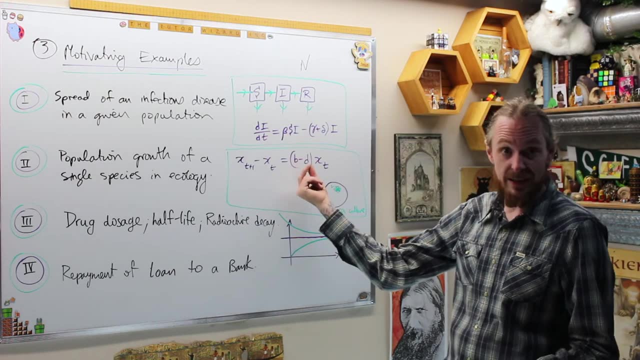 culture is going to be with when we're in the petri dish. there's no migration in or out, So it's a closed system. we're assuming, And so we're going to be. if we have a birth rate and a death rate, we're going to assume that that's positive. So then it's going to grow, And the difference 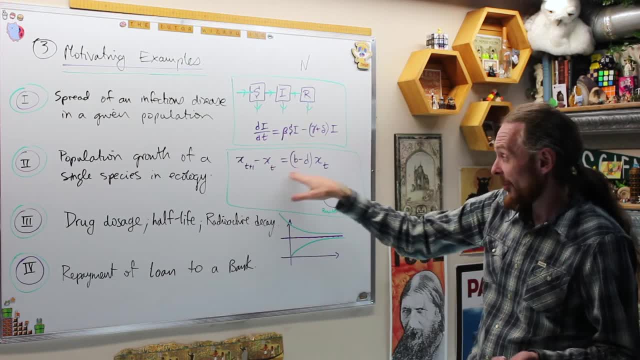 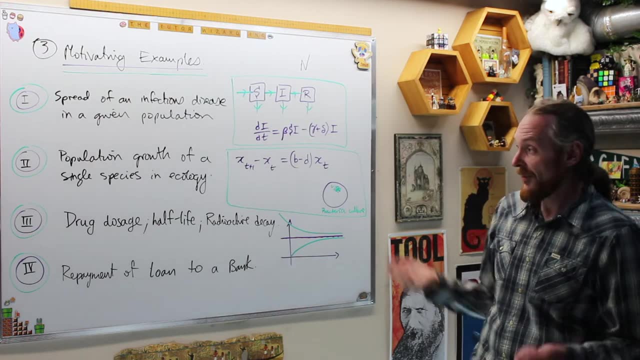 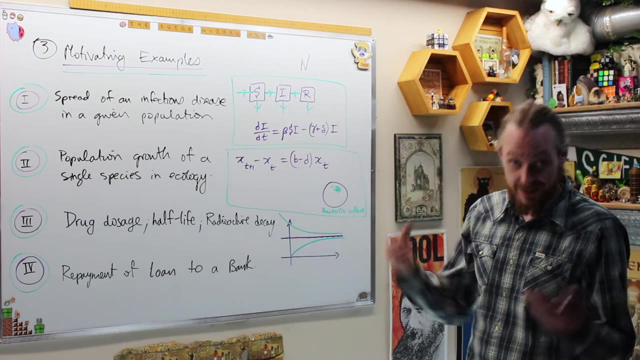 between those changes in the generations. populations is going to be directly proportional to the population at the original generation, And this is a difference equation that we can build from population growth. we can also do the continuous version, So this is a continuous modeling of some. 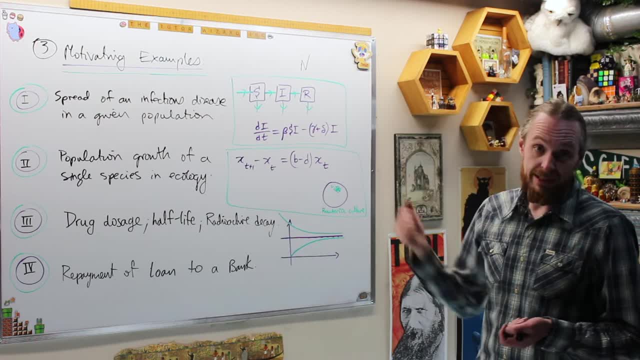 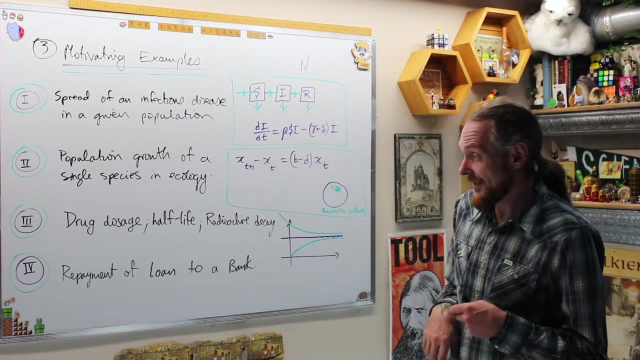 scenario in the world- And this will be a discrete one And a couple other ones that we're going to do throughout the course and I'll probably give assignments or those types of things or discuss in detail is going to be the notion of exponential one. So if we have drug dosage and half life in 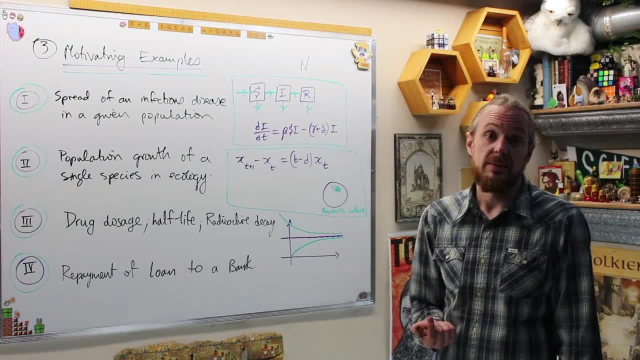 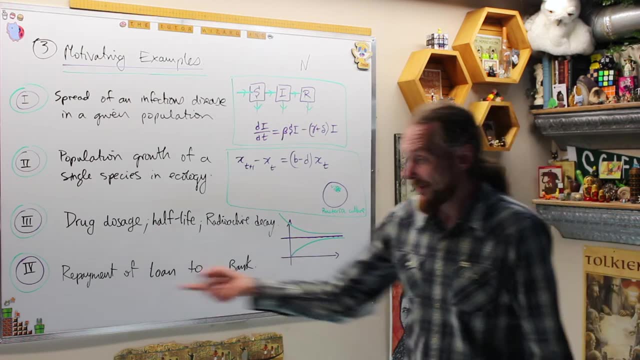 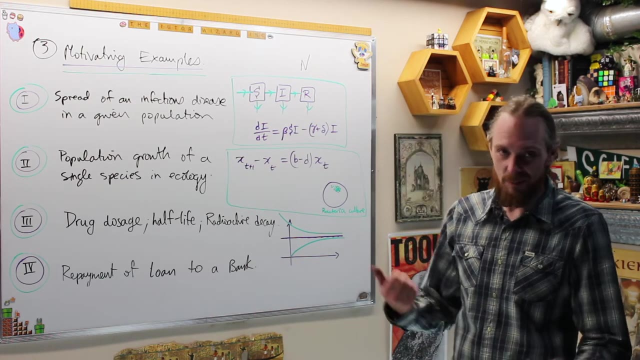 the bloodstream or half life of radioactive decay of certain materials. we're going to get a way of both discreetly and continuously modeling these things And maybe you don't want to know, but a lot of people have been doing some research into how to do repayment- monthly or yearly repayments of loans. 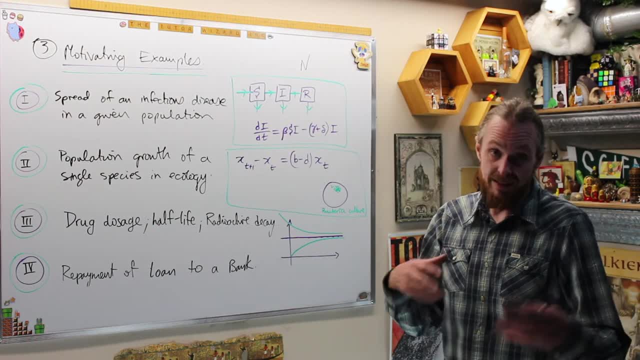 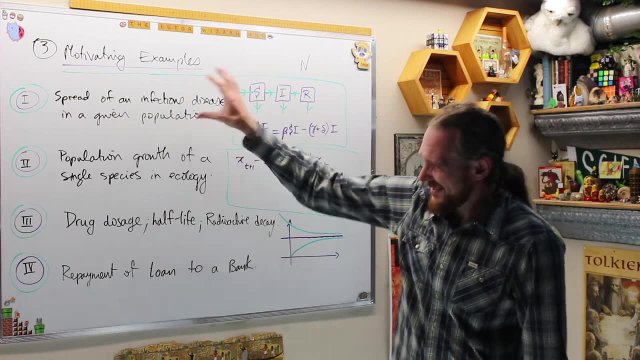 to a bank. How do we model this repayment And how do we get an explicit function to predict how these types of things are going to go? So these are the four main models- the two that I'm going to consistently look at are going to be spread- of infectious disease models and population models. Let's do number four. 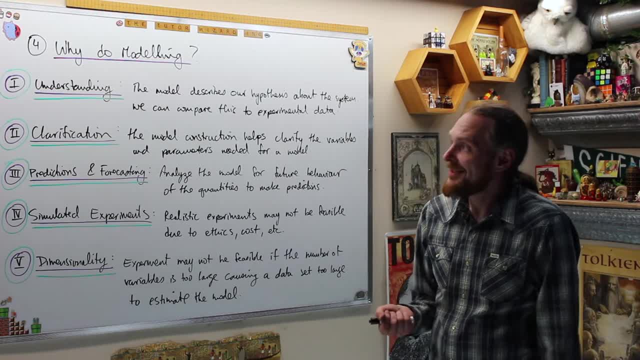 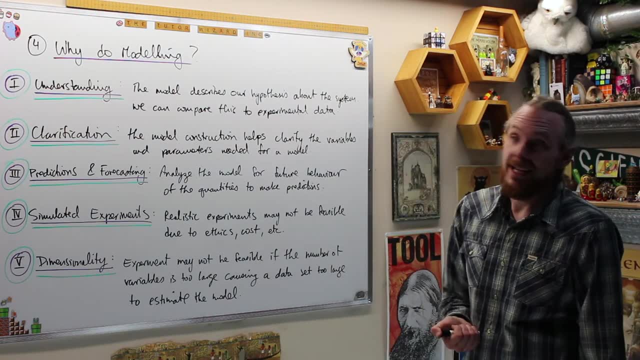 Four, why do we want to do models, Or why do it in the first place? I'm supposed to try, and just because I said so in this course, but here's some other justifications. One is going to be understanding. the model describes basically the hypothesis we have about that system Once we do. 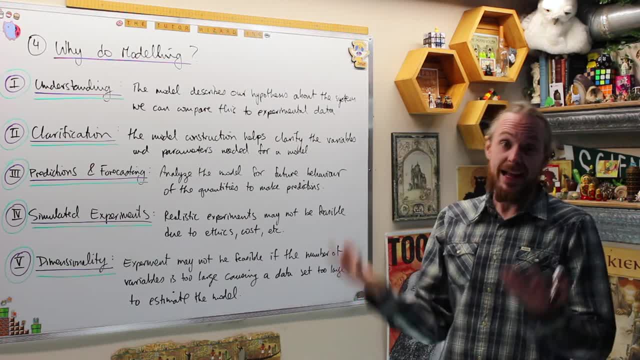 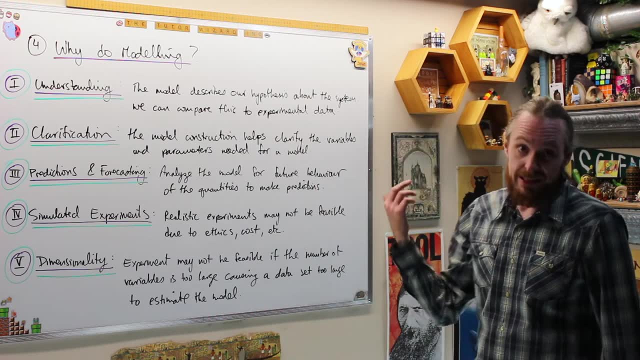 that we can actually compare this to experimental data and see if the model is actually predicting what's happening in the real world. So it will give us an idea of what's going on in the real world. It will give us feedback of whether we're doing this correctly or not doing that correctly. That's. 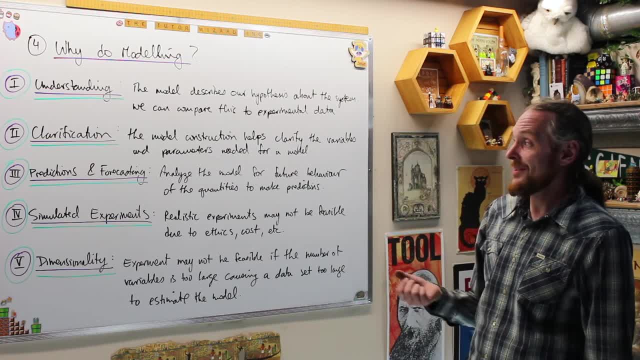 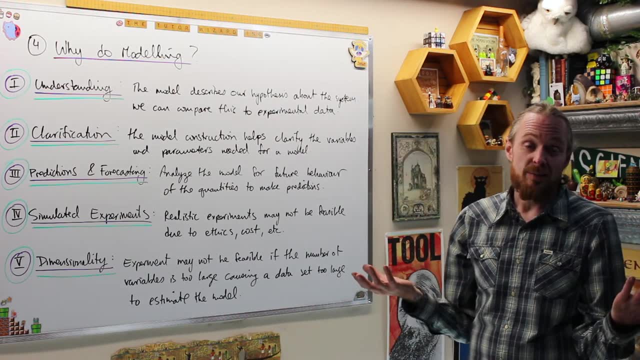 essentially what two is. that gives us clarification. Once we can do this, the model construction helps us clarify what parameters we need to keep in there and which ones we could throw away possibly, or what's important to the model to construct this and see what's going to happen for the future. 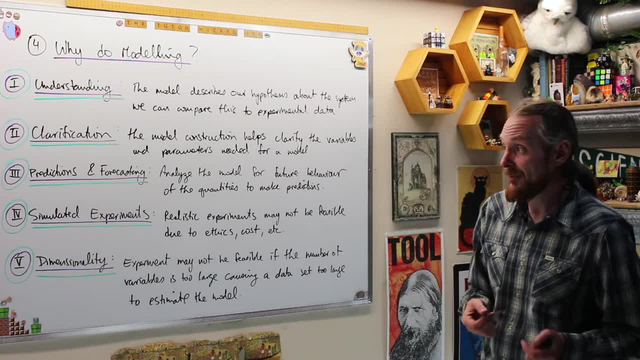 behavior of the disease or those types of things, and which ones we can leave behind. The process of actually making the model and sitting down and saying what do we need or how is that happening, actually helps quite often. So that's one of the things that we're going to be looking at. And then 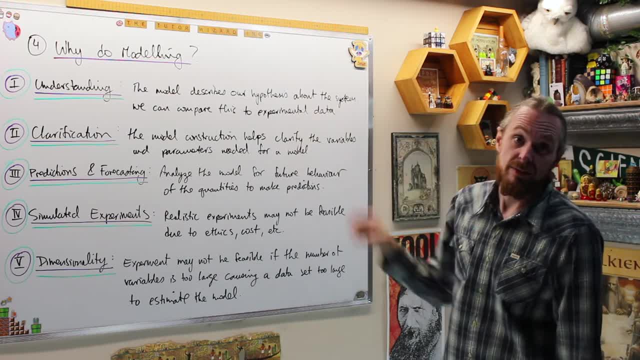 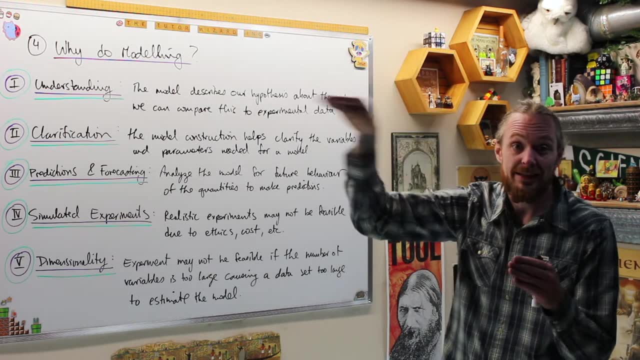 to clarify that. and then we go back to comparing to data And if it doesn't match we say, oh well, that's unrealistic. Populations just don't grow indefinitely unbounded. There must be a carrying capacity. And how do we add carrying capacity in the model? We have to tweak the original equation. 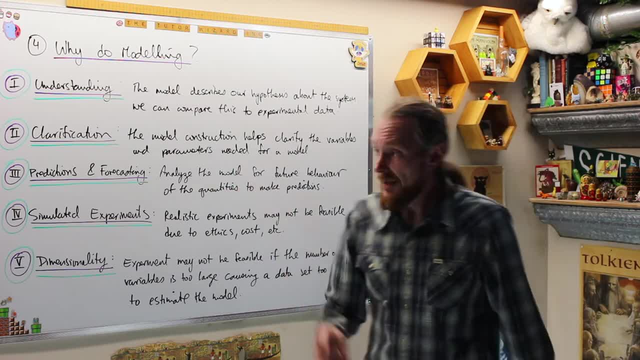 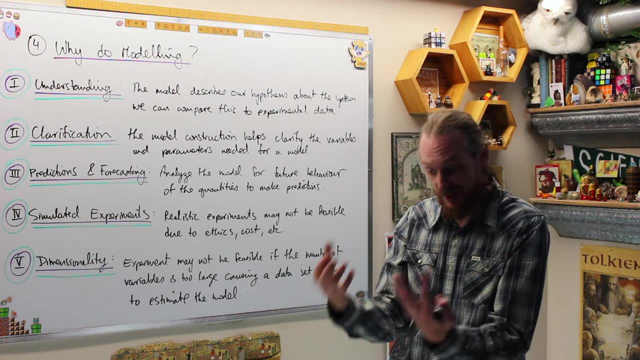 somehow, And we'll do that throughout the course. The other thing it's good for is predictions and forecasting. The whole point is, once we're good at setting up the model and finding the solution to them, whether they're analytic or when they're complicated and nonlinear, we might have to use 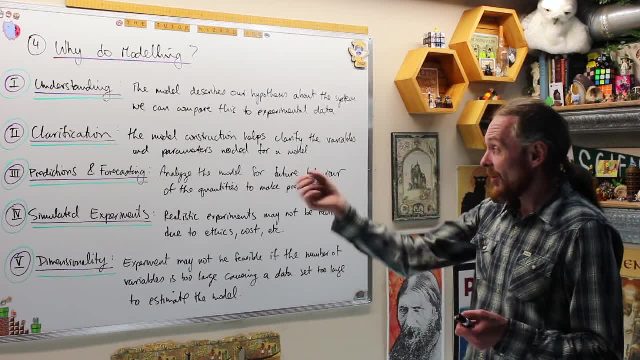 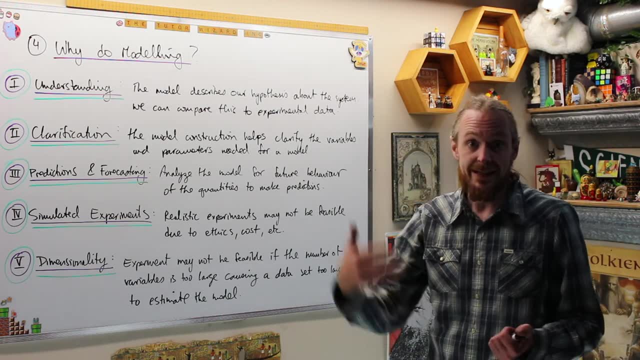 numerical solutions. But either way, once we have that, we want to analyze the future behavior of these quantities so that we can make predictions or try to mitigate through quarantine or inoculation vaccinations of a certain disease. That's the idea. We want to model it and then 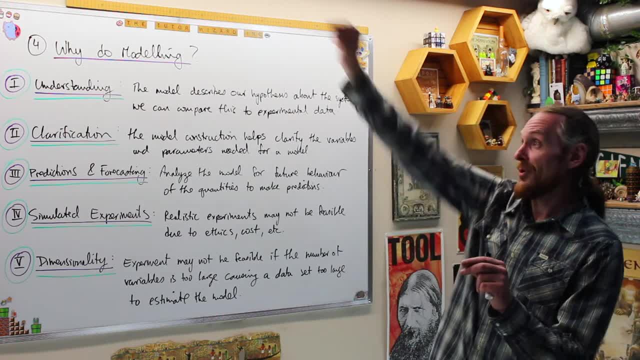 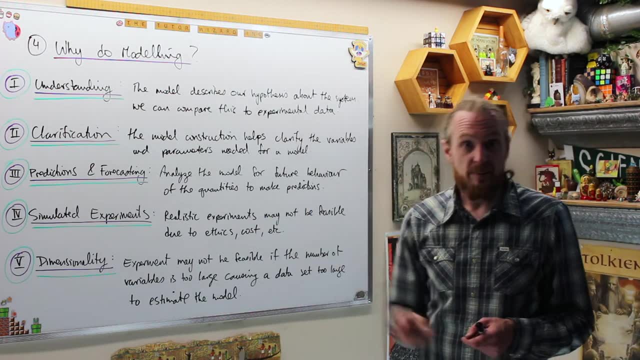 analyze that to say, hey, the disease is going to do this, or it's just going to, everyone's going to get it, or it's going to die off soon, or what's the tipping point. And we want to analyze these types of things, Also some things that people don't think about until you point them out. 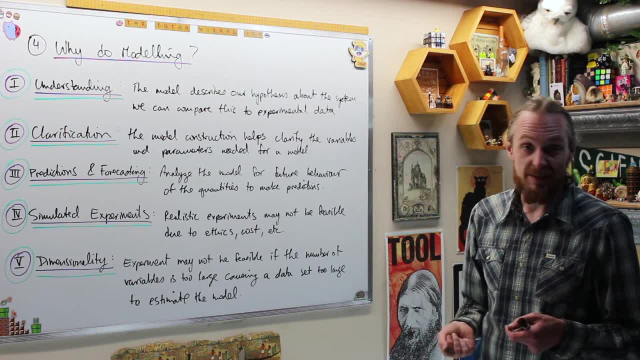 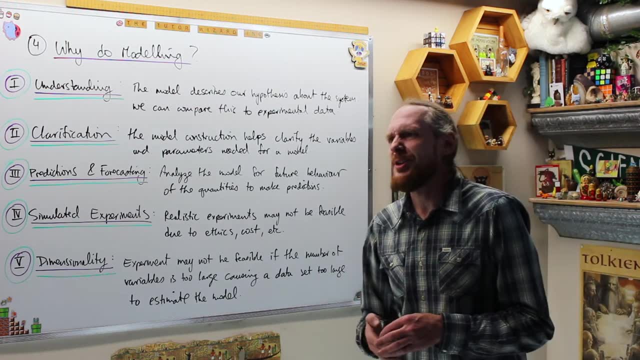 but it's simulated experiments. A lot of the time, realistic experiments in the real world can be feasible due to ethics or cost or those types of things, And it's like: well, which ethical ones? It was like: OK, I want to know, I'm going to give you a drug dose for your certain kind of condition. 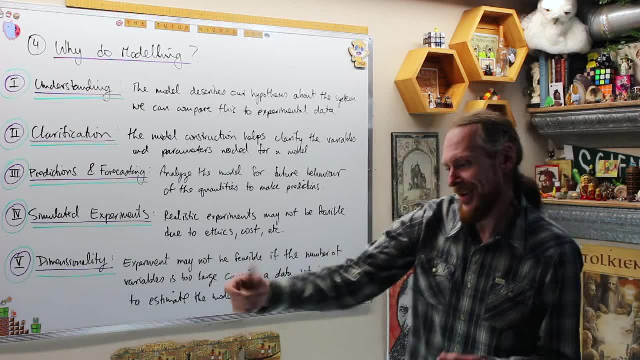 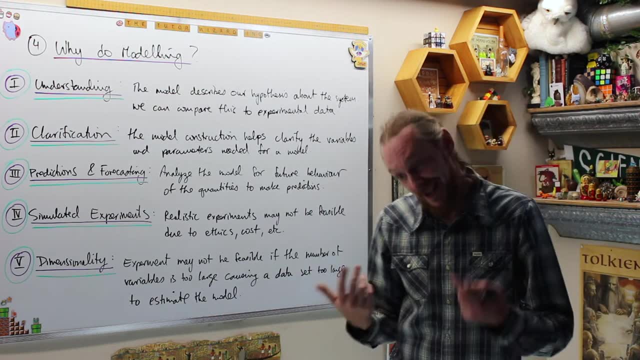 that you have. But if I give you too much you die. I can't just keep giving you amounts until I'll be like, oh, that was enough, That was too much, And then just start easing back from death to be like which was the correct dose. So that might not be a good idea. Or if I have some kind 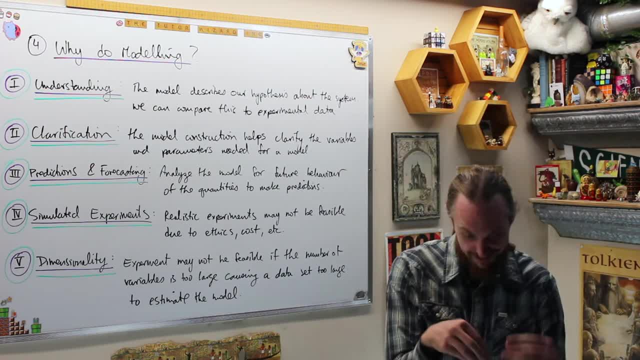 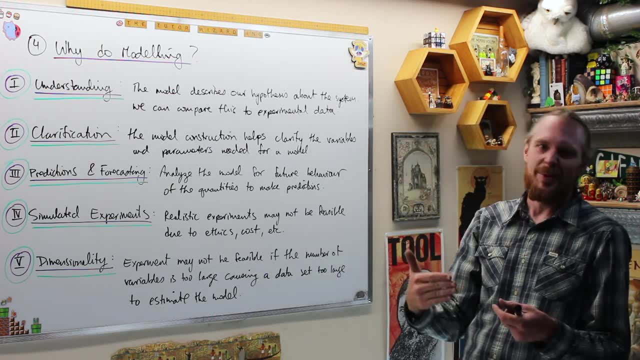 of toxic Marie Curie? she's like I found radiation. She's like I found radiation. She's like I found radioactive stuff. And then yeah, a few months later she's dead because she gets too much exposure. We want to know what's a good amount of exposure, what's too much exposure. We can't. 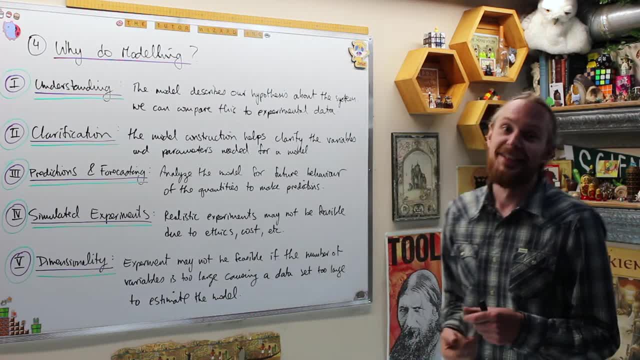 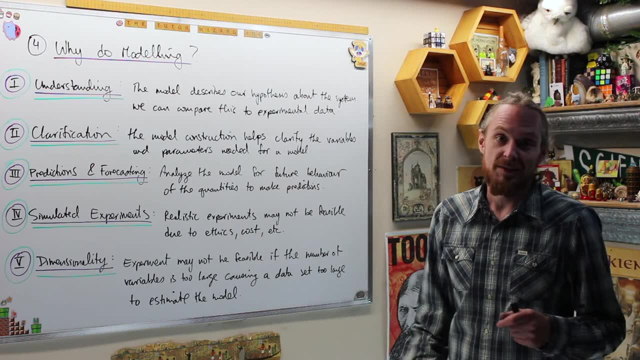 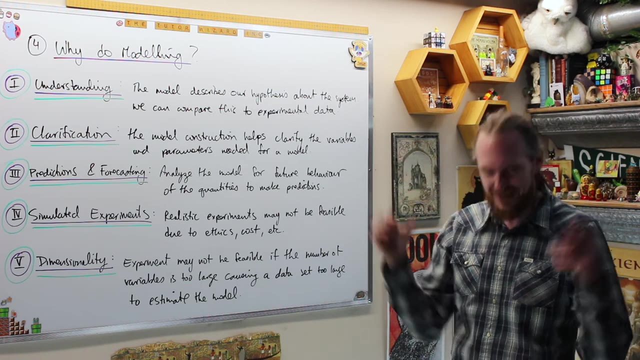 just keep giving people. ethically We can't. just keep giving people. We could, I guess, But in ethical scenarios we can't. Another good motivator is cost. If you actually had to try to somehow get some kind of data from every individual in the world, how are you realistically going to A 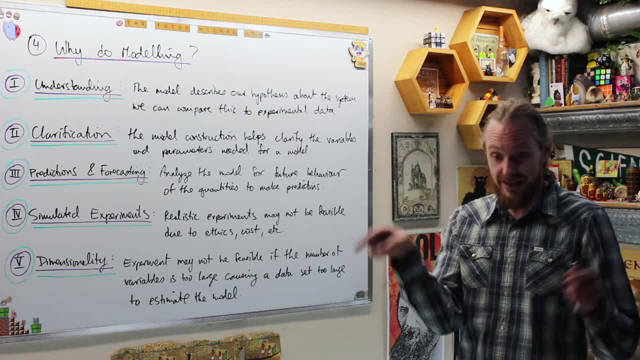 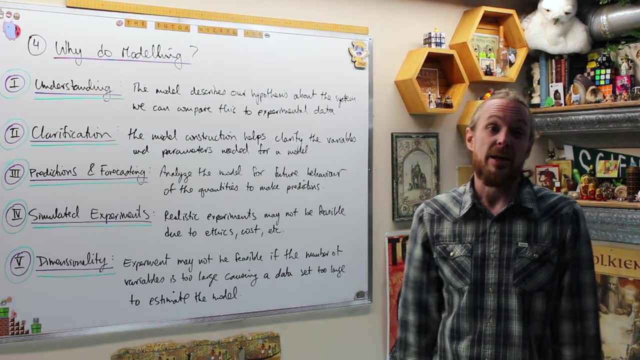 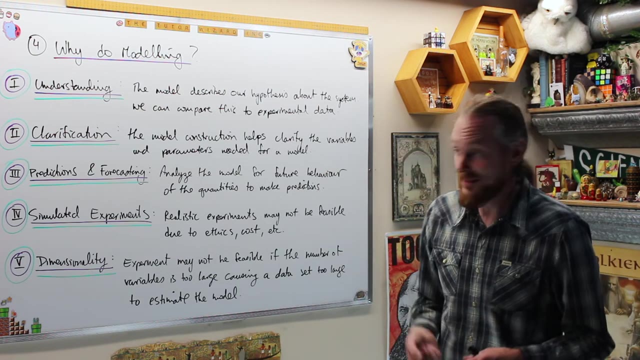 get that and B afford to do the survey or get someone to go around and do that, So cost and the physical world will often create scenarios where we can't actually run the experiment. So on the other hand we can. if we get accurate models, we can put it into a computer and run all kinds of different simulations. 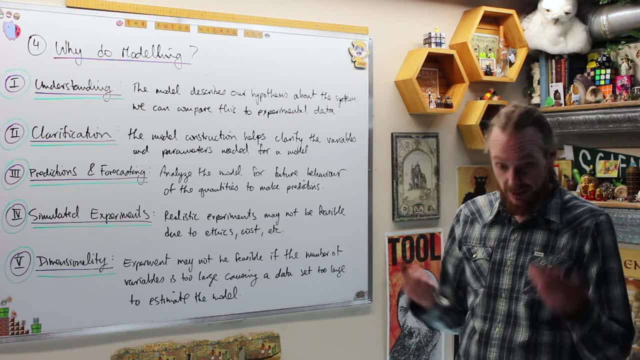 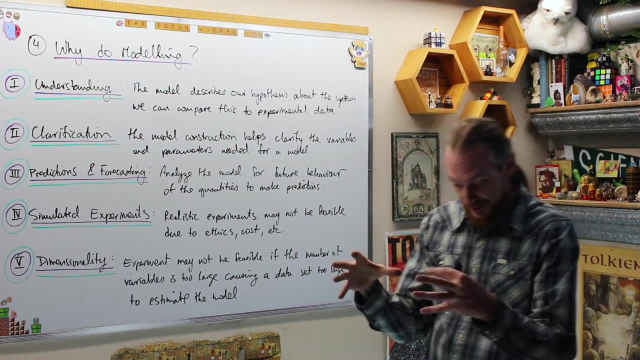 And that's relatively cheap in comparison to some of these ethical or cost scenarios. And then the curse of dimensionality, Eventually, if we have too many parameters. that's why we're going to start off with small models and then make them more and more accurate as we go And we'll see. 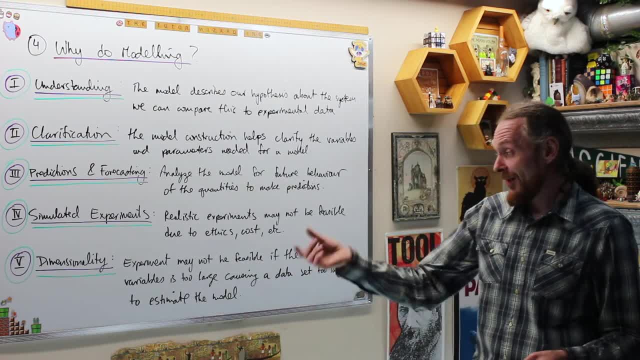 how much more complicated it's going to be in the future. So that's one of the things we're going to be trying to do, And the other thing we're going to be trying to do is to solve them. Once we have so many variables that it would cause such a large data set, we can't accurately estimate the. 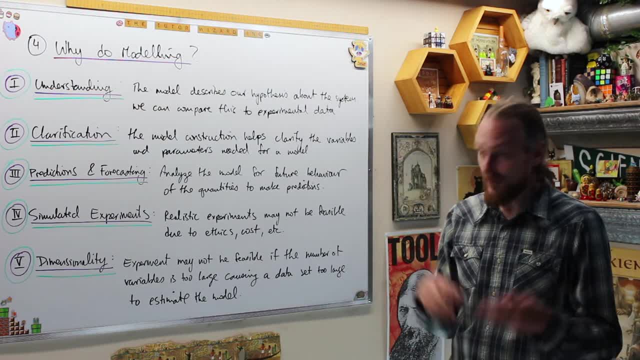 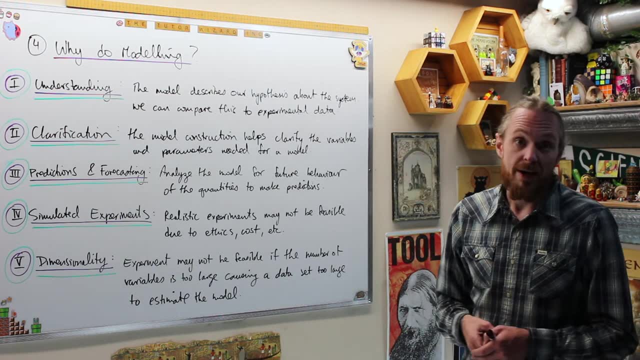 model in the real world, So we wouldn't be able to collect enough data, So we can't actually run the experiment again. So computer programs are cheap and we can make the computer program run it a bunch of times and see what's going to happen there and use predictions. So these are the 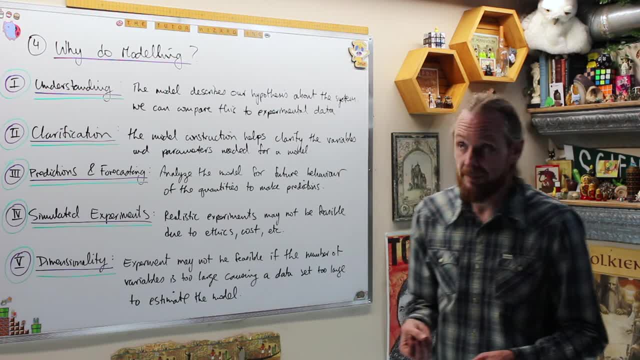 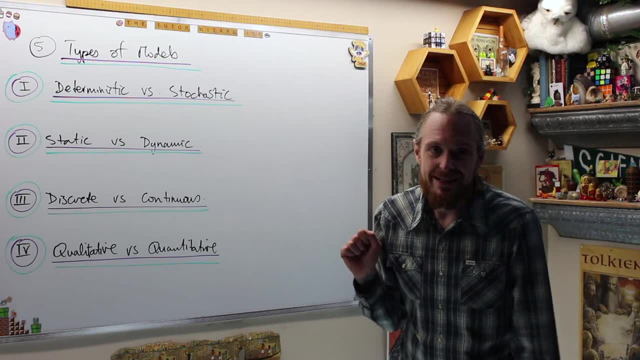 motivating reasons as to why we would want a model in the first place. Let's do number five, which is the different kinds of models that we're going to do. Part five is going to be the types of models we're going to deal with, or, in general, that you can consider. There's the first. 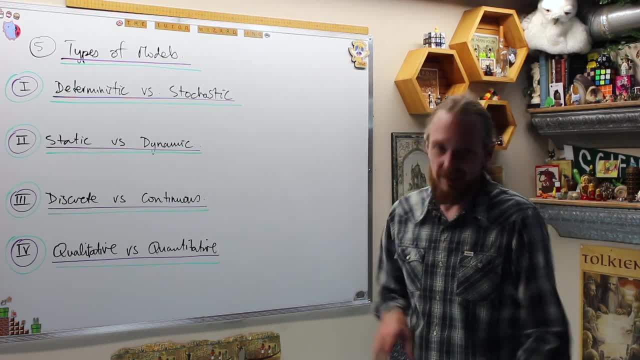 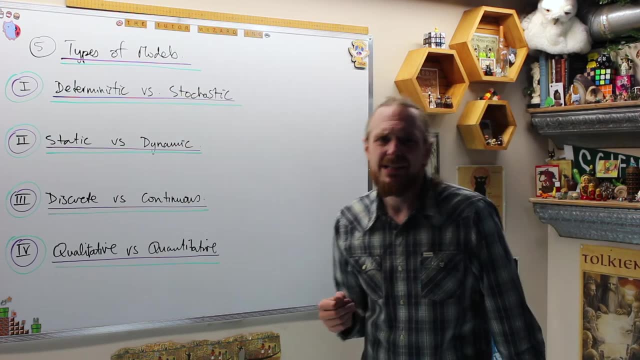 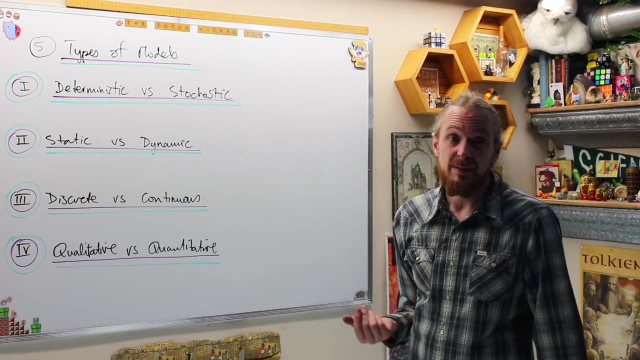 category is deterministic versus stochastic. We're going to exclusively do deterministic, mostly because this is my specialty, but you can also do stochastic. What is the difference between them? Deterministic means that the parameters don't involve any probability distribution, So there's no random chance or probabilities involved in them. Stochastic obviously means that some of 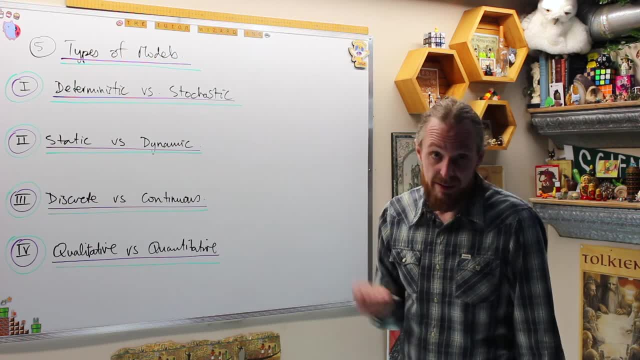 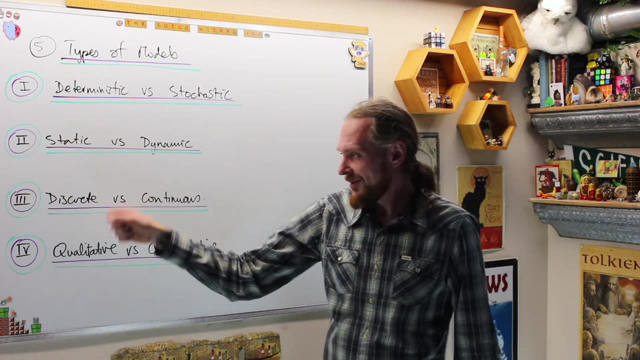 the parameters, or all the parameters, do have this probability distribution involved in them. inherently Static versus dynamic. Obviously, we're going to do dynamical systems, but in each of the two different, in these two categories, we will distinguish between static states and dynamic. 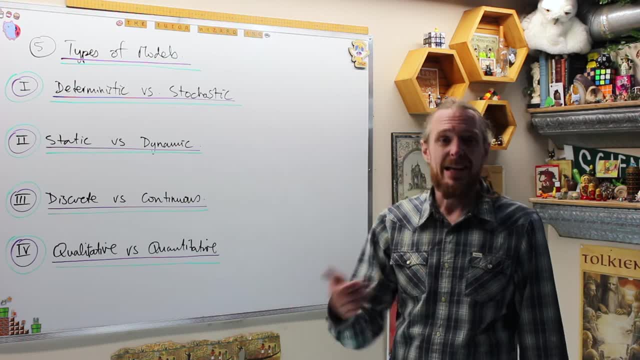 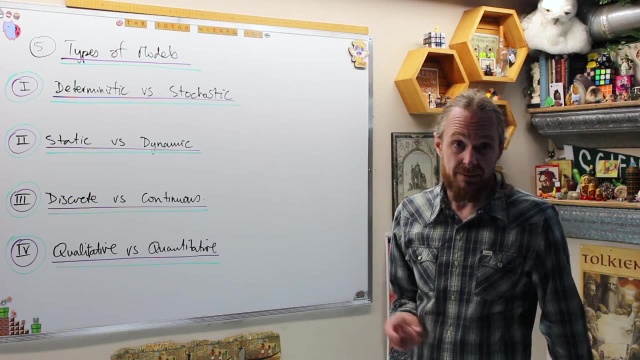 states. So obviously a static state or a steady state or an equilibrium is where we have no change in the system and a dynamical state is where we do have change over time in the system. We want to know and analyze the differences when those things happen in the models For discrete versus continuous. 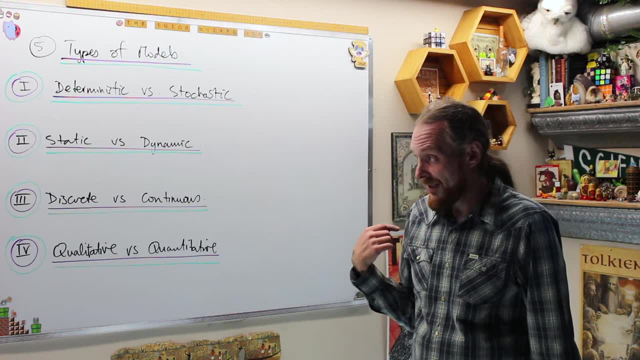 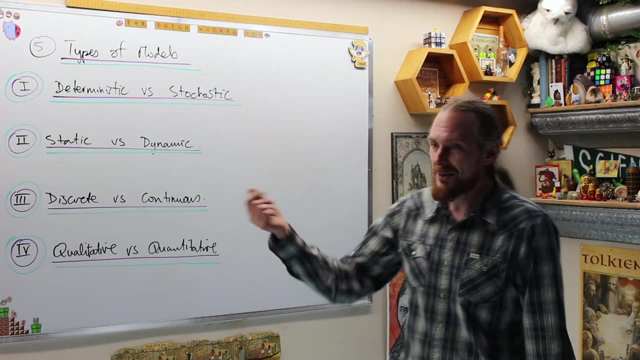 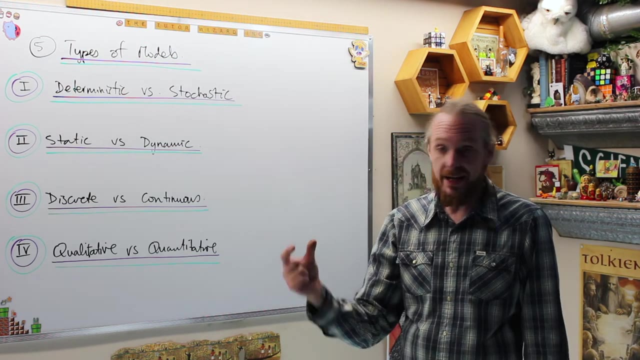 my specialty is continuous differential equations to mathematically model things. but I also like to do discrete because these are essentially recurrence relations. There's a one-to-one correspondence between these anyways. So discrete means that we have a fixed time interval, like the petri dish, and we're going to check every day, or every 24 hours. We're going to check and record. 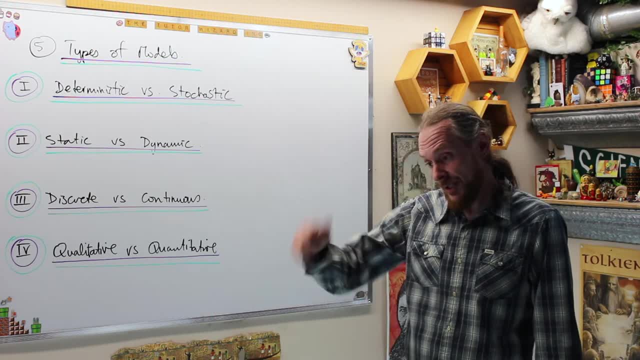 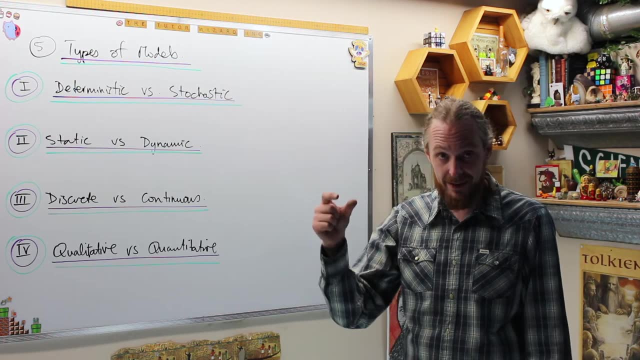 what the population is and then if we're calling that a generation, from generation to generation or from timestamp to timestamp, we will analyze this and we will have a discrete number of values in every. You can't check the population at any specific time. You have to wait for that time. 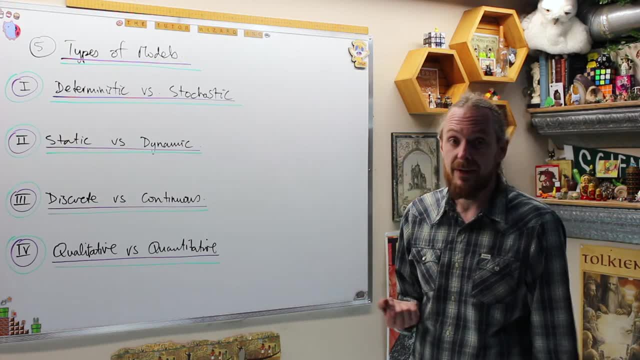 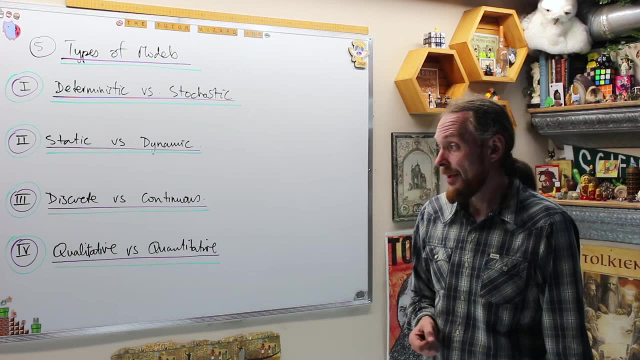 interval and then check For continuous. obviously we're going to have that. we can analyze the population or whatever. we're analyzing the process at any given time in a continuous interval. And then qualitative versus quantitative: we're going to obviously explicitly do quantitative. 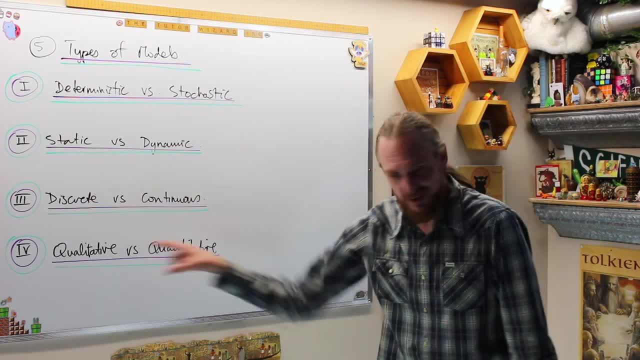 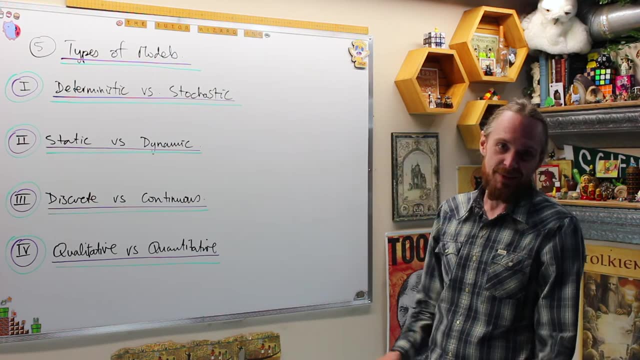 not qualitative? quanti, qualitative- I pointed again at one of these guys. who is who? Everybody hates them. Why are they? shouldn't one start with a p and one start with a q? Quantitative and qualitative. that would make it easier for me a little bit. but 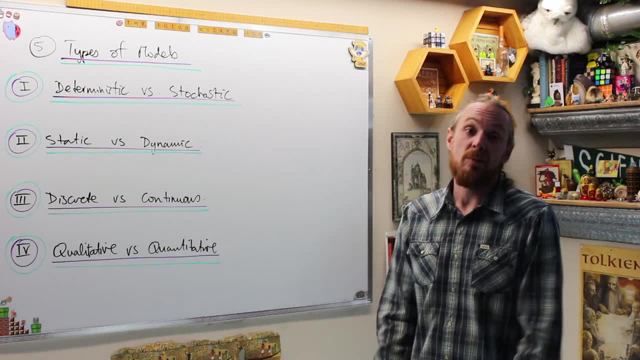 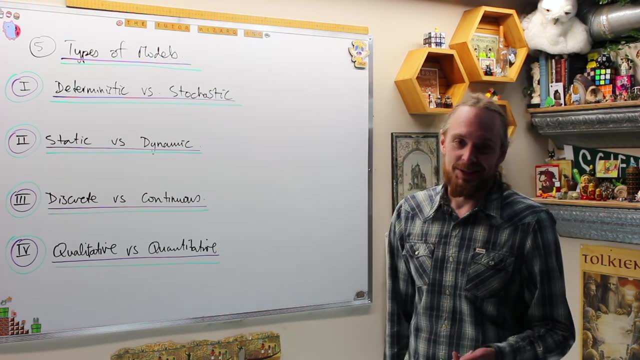 qualitative means it has to do with something that we can't measure but we can observe. A really good example of this is not a real science, I'm just kidding- but linguists and language. It's something that you can observe, but we can't empirically measure it in any way.